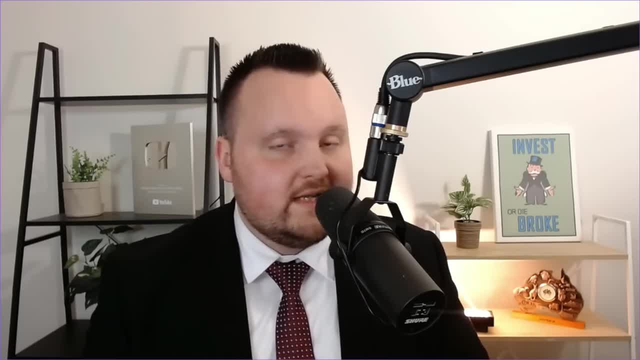 do or what nobody thought would happen so soon. So in today's video, we're going to go over exactly what's happening with used car prices, Because, people, this has been an absolutely crazy mania bubble. Used car prices have been rising 50% year over year. This has been driven by record. 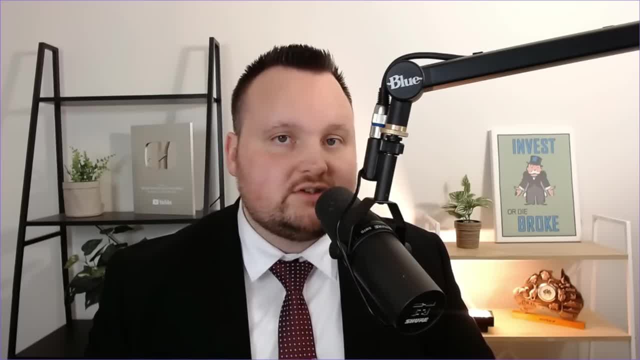 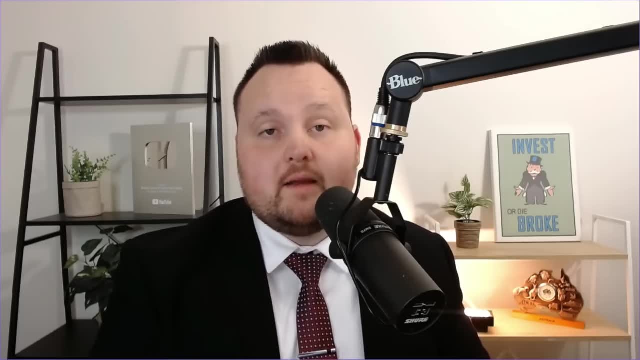 low inventory, supply shortages, factories being shut down and records amount of stimulus during 2020 and 2021.. But all the ingredients that fueled this used car market bubble is now going into reverse, especially lending, with interest rates going so high. So if you've been one of those, 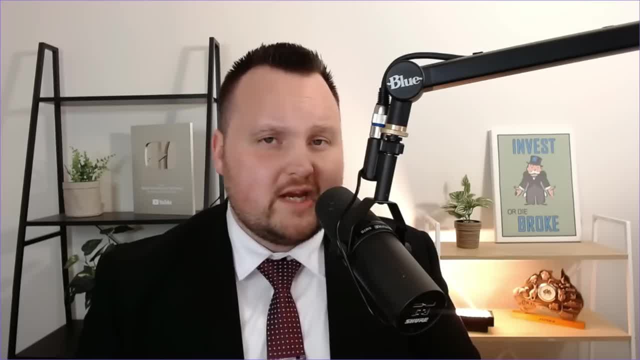 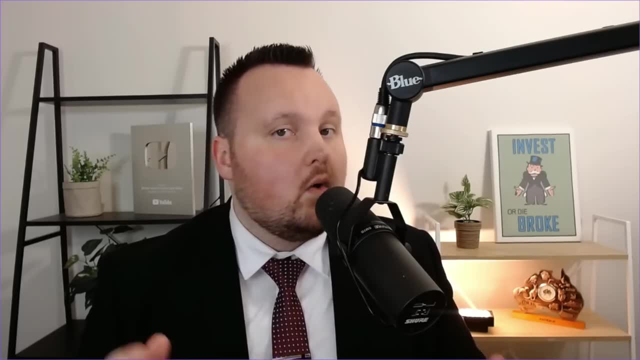 frustrated buyers for the past two years, being unable to negotiate with car dealers. well, dealers are about to be in a world of pain. So everyone, what exactly is happening with used car prices And what's happening with used car prices In the used car market? where is it going to go? What should we do? Will there be some bargains? 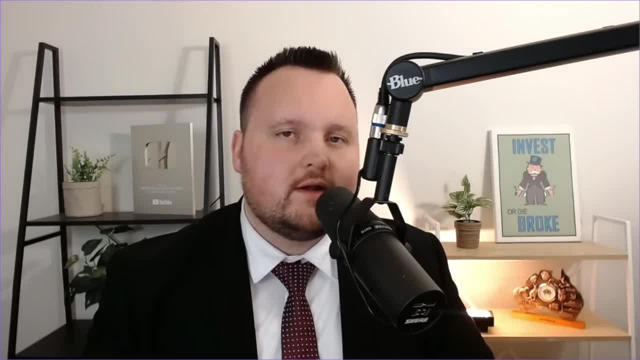 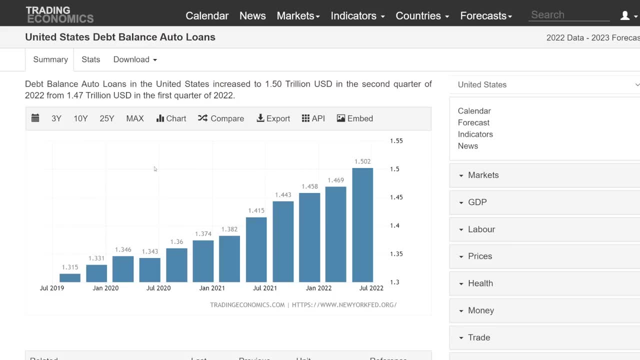 coming very, very soon, Could you get that dream car you've always wanted. Well, let's not waste any time, ladies and gentlemen. Let's get straight into the news, the facts and the data. Okay, So, first things first. look at this: This is the auto debt balance We can see here, since 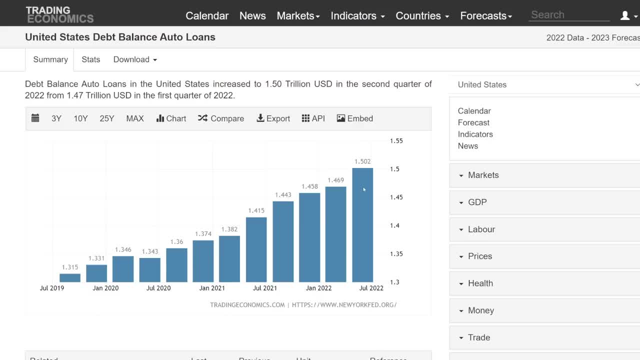 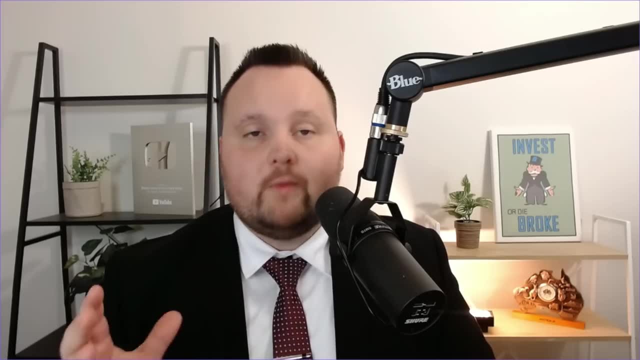 July 2019,. it has been absolutely skyrocketing and has just hit a new record, as we can see here, of 1.5 trillion And, with auto loan debt, a record highs, right when interest rates are rising rapidly. this is a recipe for disaster, Because 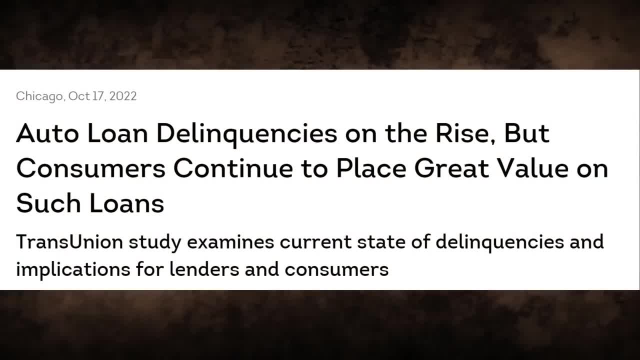 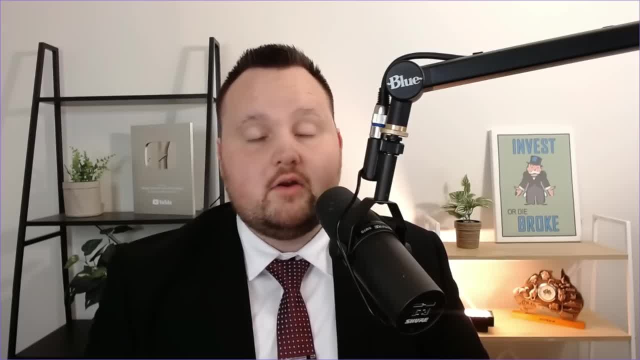 look at this everyone, And this is just the first piece of the puzzle- Auto loan delinquencies on the rise, but consumers continue to place great value on such loans. So while, yes, consumers do put a lot of value on their car loan, the mortgage comes first, And what's happening with inflation is cost. 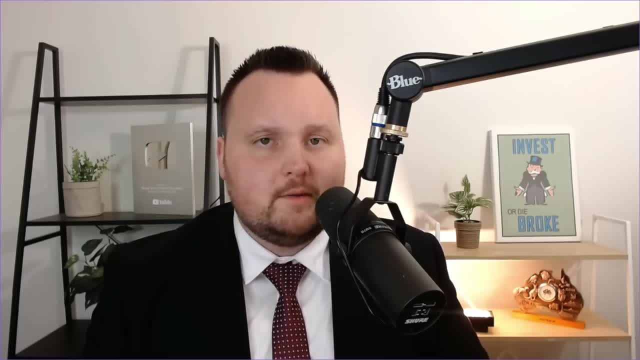 of living is rising rapidly. People can't afford to heat their homes. They're going to barely afford their grocery bill, So they may be forced to sell their cars and downgrade to keep up with the rising cost of living, And that's a recipe for disaster. So let's look at this: everyone, And this is just 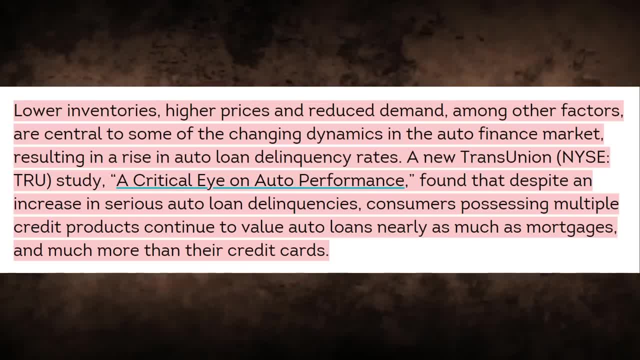 the first piece of the puzzle. We can see here: since July 2019, it has been absolutely skyrocketing and has just hit a new record. We can see here since July 2019, it's cost of living is rising rapidly. People can't afford to heat their homes. So let's look at this: everyone And this. 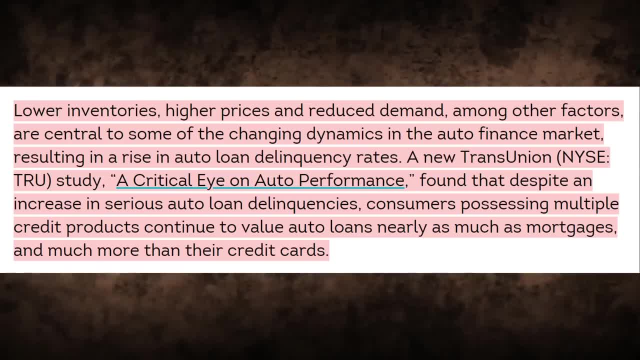 is just the first piece of the puzzle. People can't afford to heat their homes, So let's look at this among other factors essential to some of the changing dynamics in auto finance market, resulting in a rise in auto delinquency rates. A study found that, despite an increase in serious 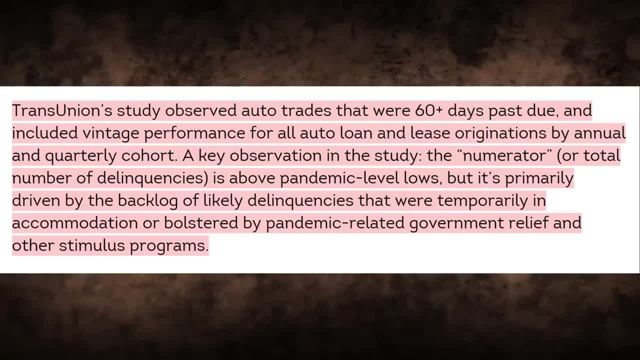 auto loan delinquencies. they observed 60 plus days past due and included vintage performance for all auto loans and lease originations by annual and quarterly cohort- A key observation in the study: the numeral or total number of delinquencies is above pandemic lows but is primarily driven 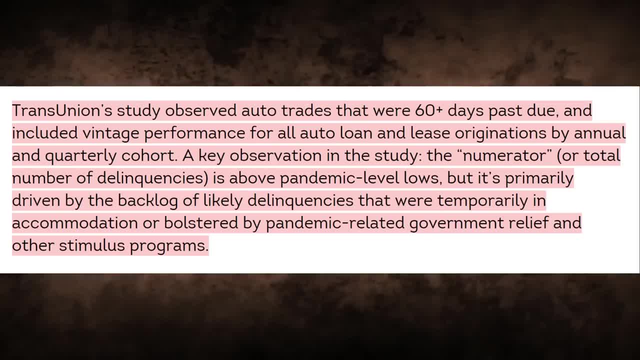 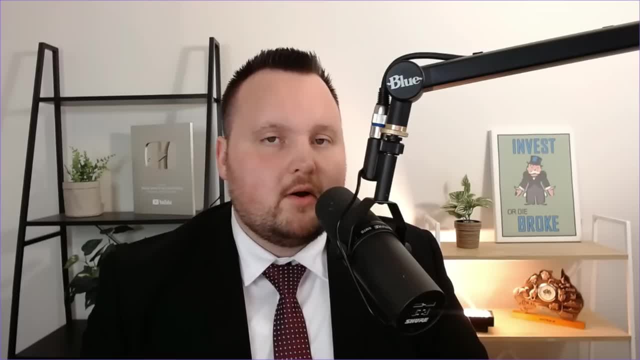 by backlog of likely delinquencies that were temporary in accommodation or bolstered by pandemic related government relief and other seamless programs. So that is right, everybody- The banks- put a lot of repos on hold during the pandemic, kind of like how people didn't have to. pay their mortgage, either during the pandemic, because they didn't want the banking system to collapse. But now that things are coming back to normal again, the banks are coming knocking and they're starting to say: look, it's time to pay up or we're going to take your car. 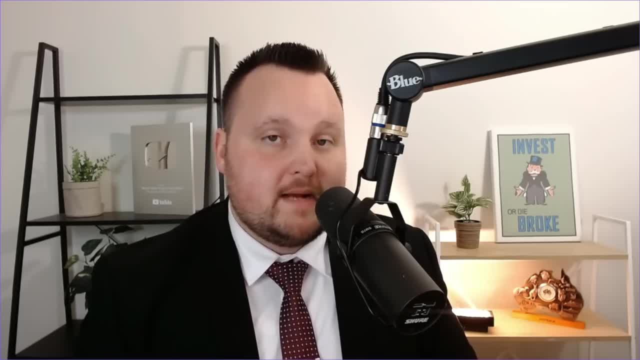 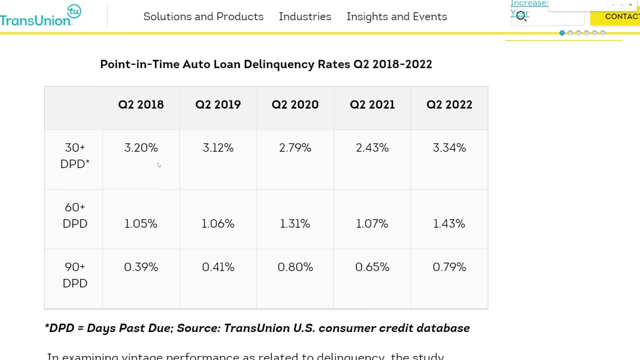 Especially, they're worried that car prices may start falling and start affecting their balance sheets. But look at this here: This is point in time: auto loan delinquency rates due to 2018 to 2022.. Now we can see here: 2018, it was 3.2% and now it has reached a recent high. 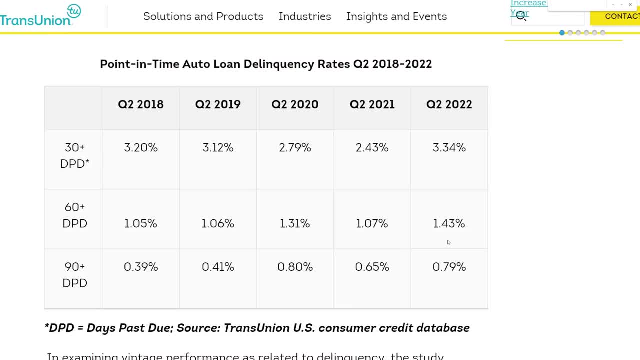 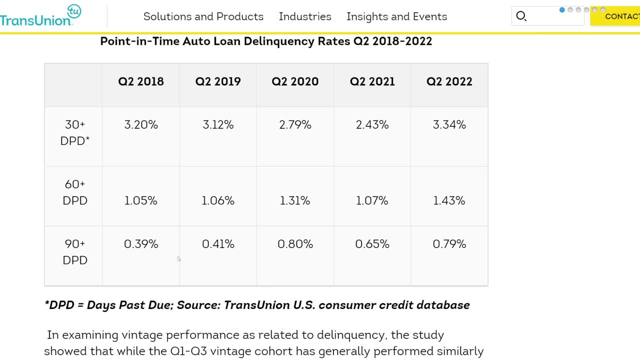 of 3.34%, That's for 30 days late- 60 days late is a record as well- from 1.05% to 1.43%, And 90 days later it's gone from 0.39% to 0.79%, And while these may not seem like crazy levels yet, 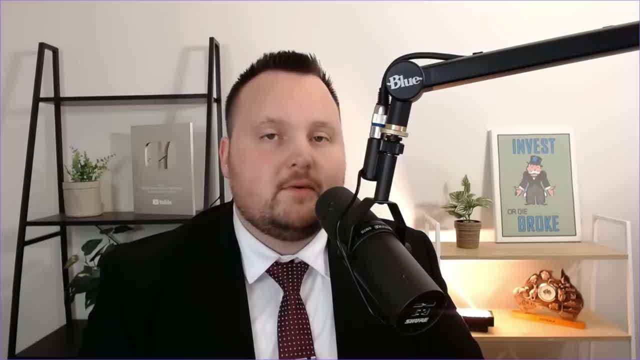 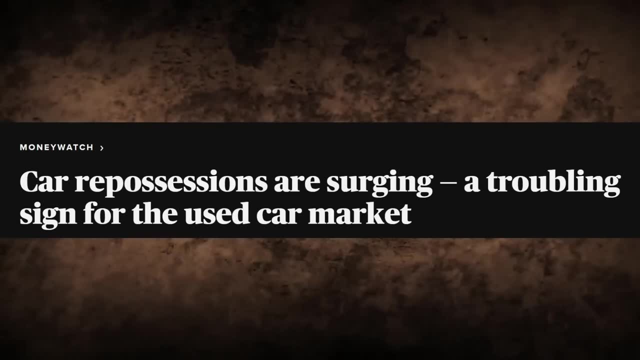 people as inflation, the cost of living crisis gets higher and higher, As people get more and more behind on their bills. it is only going to get worse And the trend is your friend. and the trend is going higher Because, like I went over in my previous, 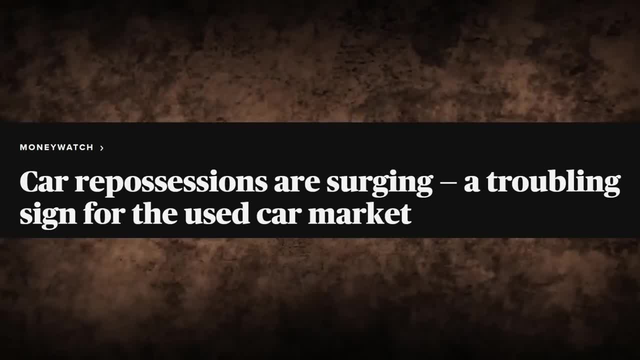 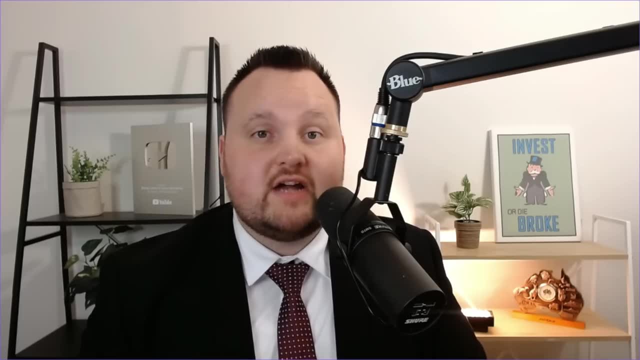 video. car repossessions are surging and it's a troubling sign for the used car market, But I know what you're wanting to know is okay. well, are used car prices falling? And people, you may want to sit down because this data may shock you. Look at this: Used car prices record largest year. 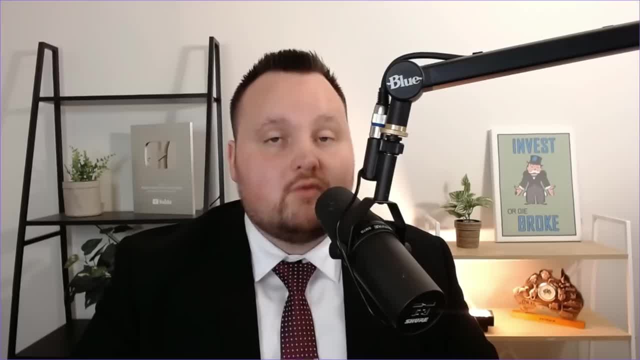 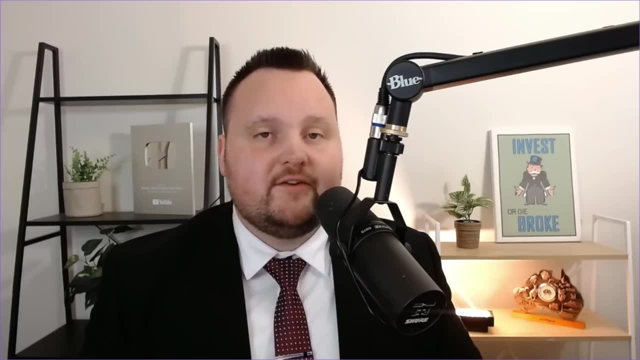 on year decline since the global financial crisis. That's right, everybody. Car prices right now are falling More than when they did in 2008.. And we're not even in an official recession yet. Guess what's going to happen when we do see mass layoffs come, when we do enter an official recession And like 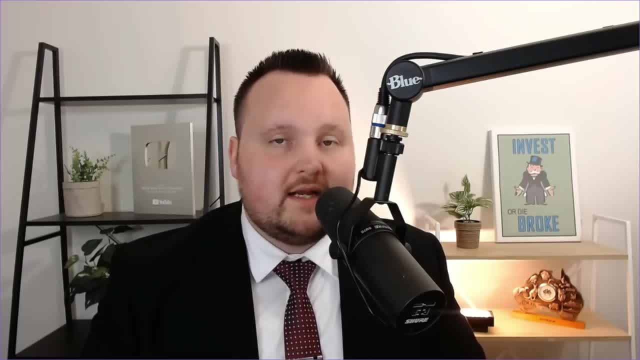 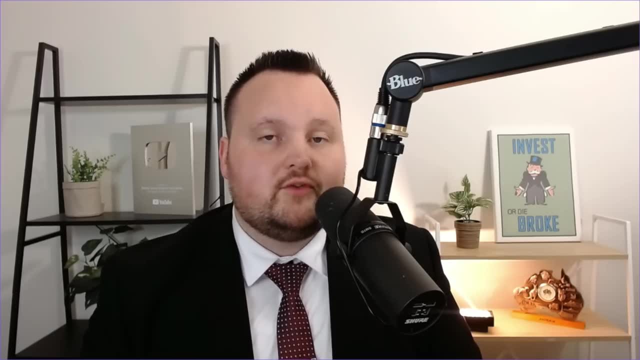 I've been thinking. I think we're going to be facing a depression If inflation keeps getting worse, the cost of living keeps getting higher. These people are going to be forced to sell their cars to pay for the bare essentials. I've also spoke to some wholesales and some retailers. 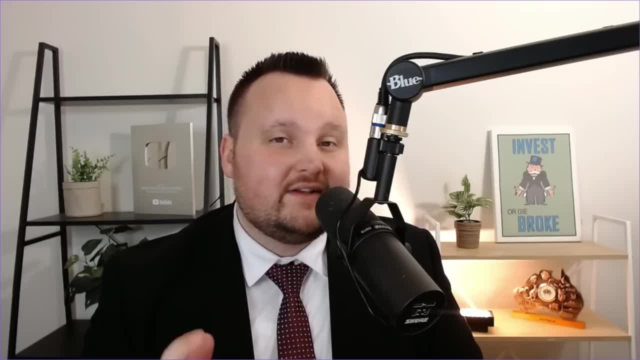 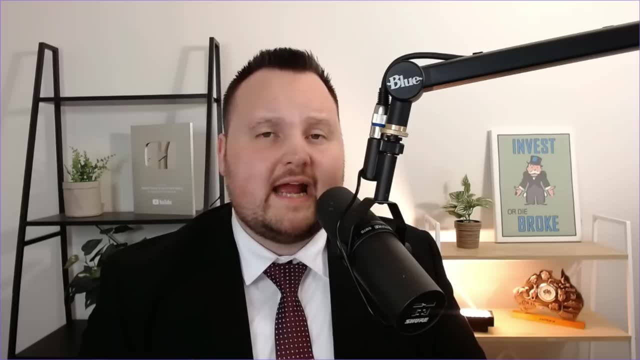 and the wholesales are saying at auctions they're seeing retailers pay less and less at the auctions- There's even been some auctions where there's been no bids at all- and have some friends in auto sales and they're saying that they're starting to have to use storage lots again because they're not able to move inventory. And I actually went past my dealer yesterday and they're literally having to park all the cars and take up all the street parking now because there's no more space left on the lots anymore. And this is happening with the RV market as well. So exactly how much are used car prices falling everyone? 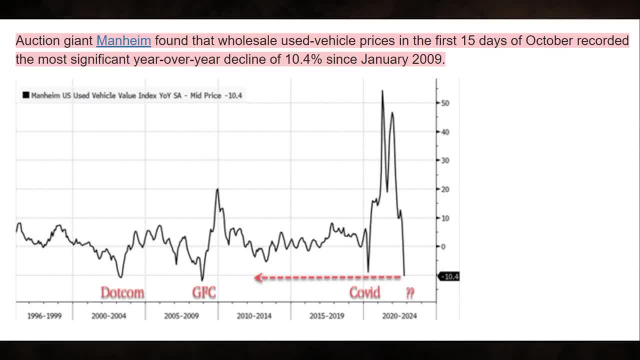 Again. this is shocking. So auction giant Mannheim found that wholesale used car prices in the first 15 days of October are falling. And they're saying that they're starting to have to use storage lots again. And they're saying that they're starting to have to use storage lots again. And they're saying: 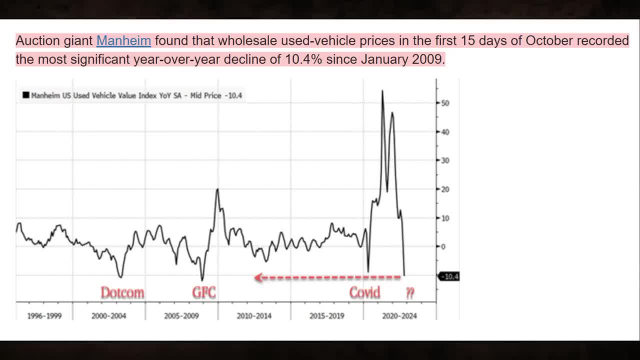 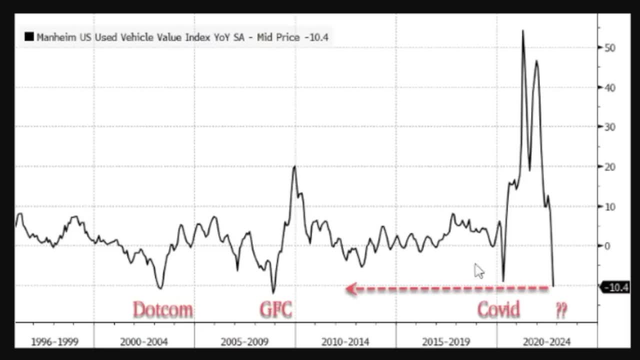 the most significant year over year decline of 10.4% since January 2009.. And look at this chart here everyone: This is a dot com, This is a GFC, This is the pandemic. And look at this down 10.4%. 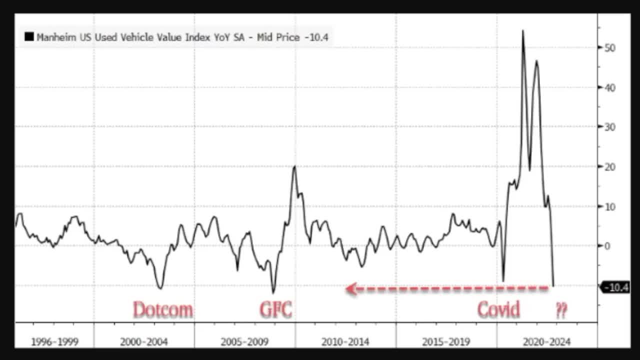 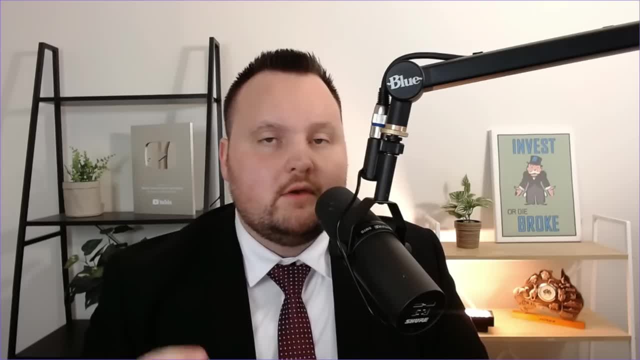 This is absolutely crazy, And it's only the first 15 days of the month. Now I still get a lot of people commenting to say that they're not seeing car prices falling yet. Well, people, this is coming from the wholesale level, So it's only a matter of time before it starts to flow in to the 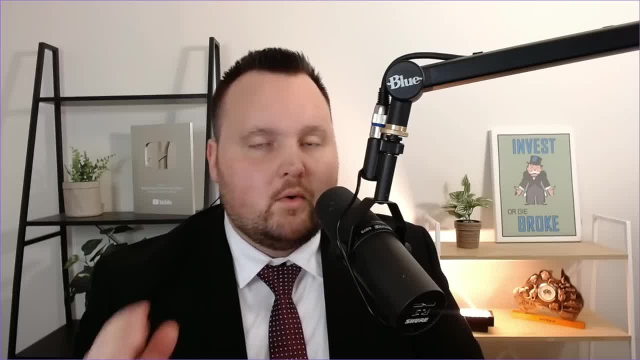 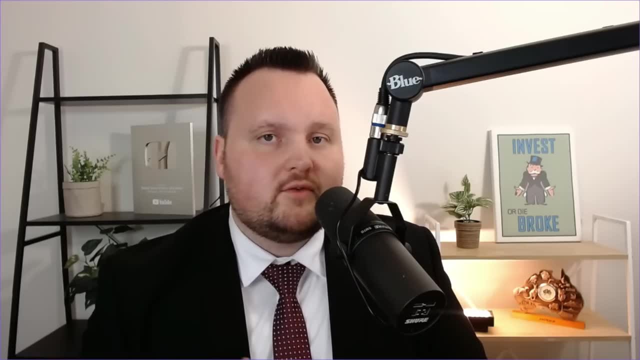 retail sector and flow into the car market. So I'm going to go ahead and show you a little bit of the chart here. lower prices in the lots, but what you may not be aware of, say, for example, the sticker price may not be dropping, but things are getting a lot more negotiable. before there was so much low inventory. 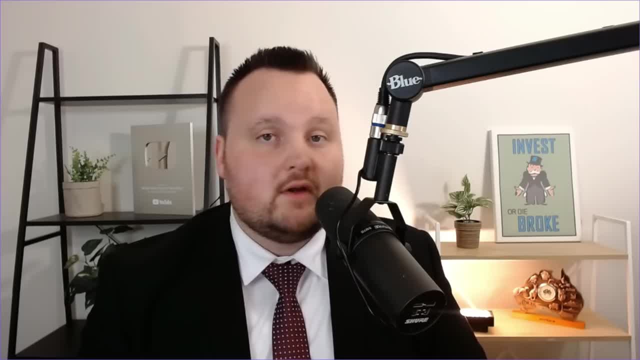 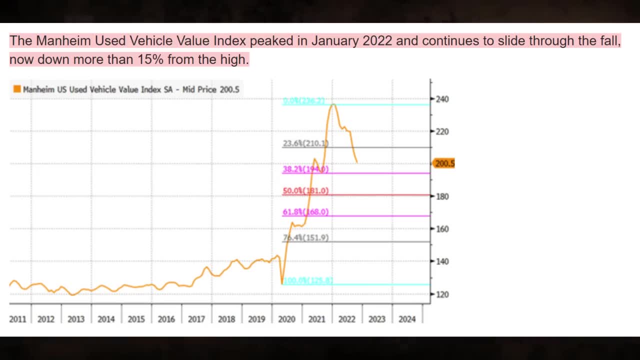 people couldn't negotiate anything at all, but now i'm sure if you go into a dealer you could be able to easily get a thousand, two thousand dollars off and get a lot more perks included. the manheim used vehicle value index peaked in january 2022 and continues to slide through the fall now down more. 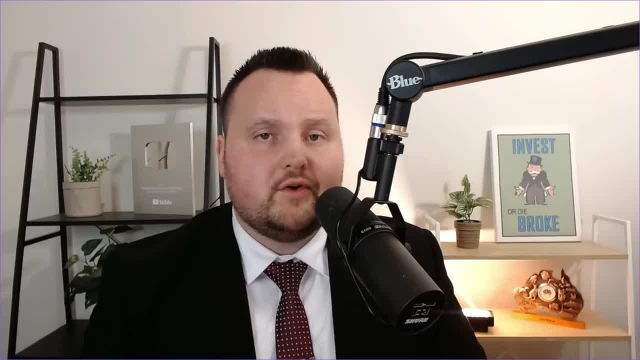 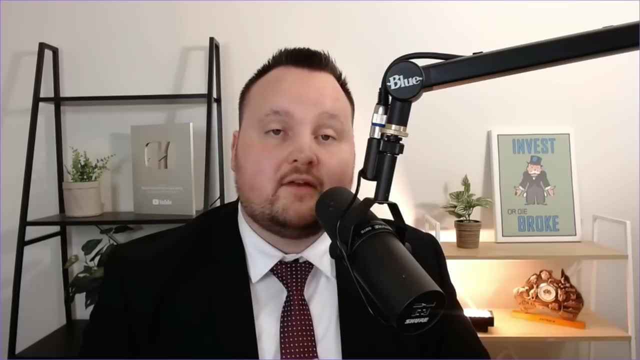 than 15 from the high. and this is not going to be the worst of it everyone. the federal reserve right now is lifting interest rates so rapidly that people haven't really felt the full impact of these higher rates. and guess what? in november they're going to do another 0.75 rate hike in. 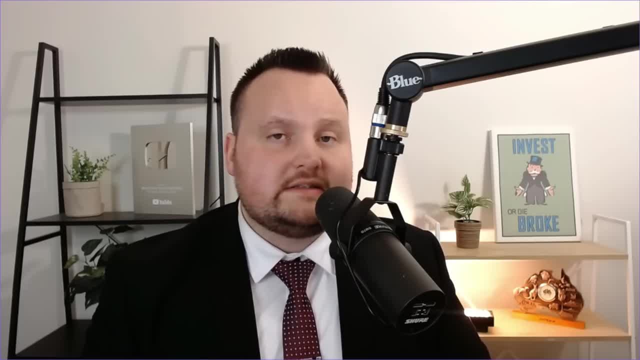 december they'll likely do another half percent or another 0.75 percentage rate hike. so we're going to see the federal funds rate over four percent and we're going to see all the loans. maybe the average rate may turn to seven or eight percent and all.